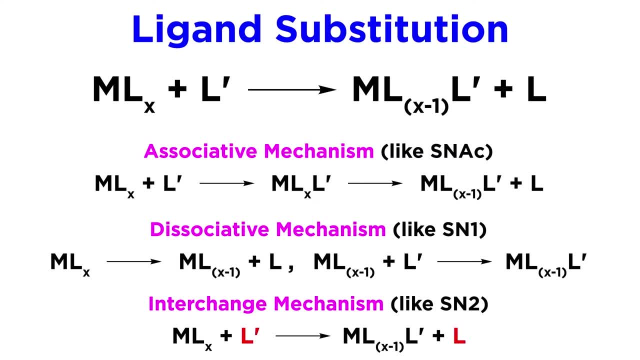 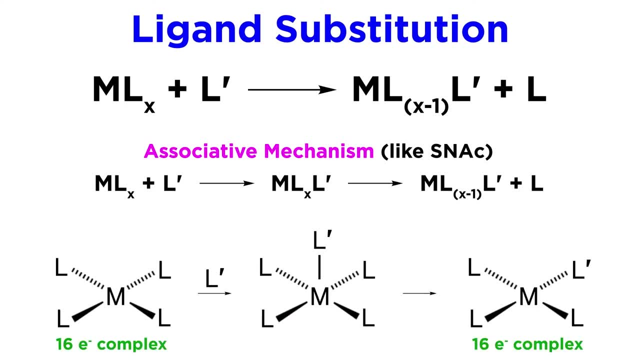 an SN2 reaction with a new ligand coordinating simultaneously to another ligand, leaving which we can call an interchange reaction. The dissociative process is preferred by 16 electron complexes, as association of another ligand forms an 18 electron complex which is stable. This is also encouraged by open 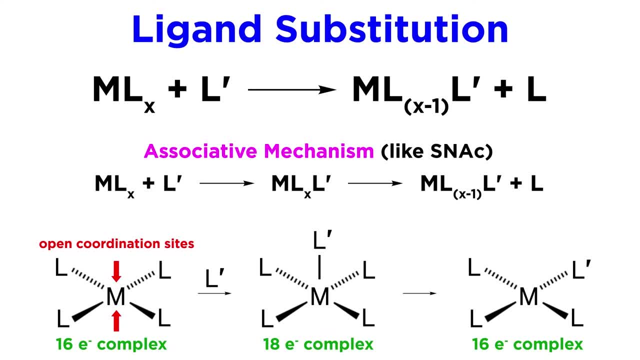 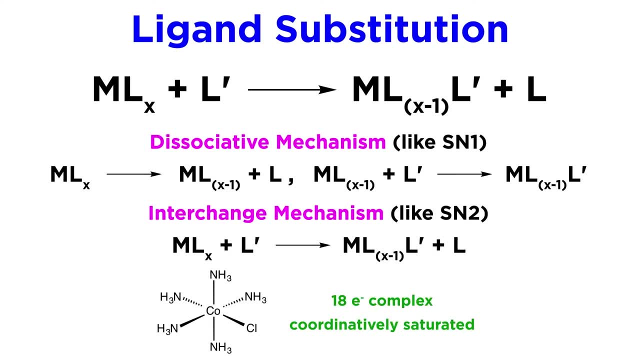 coordination sites that may be on the metal, such as with square planar complexes that can be attacked from the top or bottom. The dissociative and interchange processes are preferred by 18 electron complexes because the metal is already stable and usually crowded in terms of coordinating ligands, so one ligand must leave to make room for another, For example, 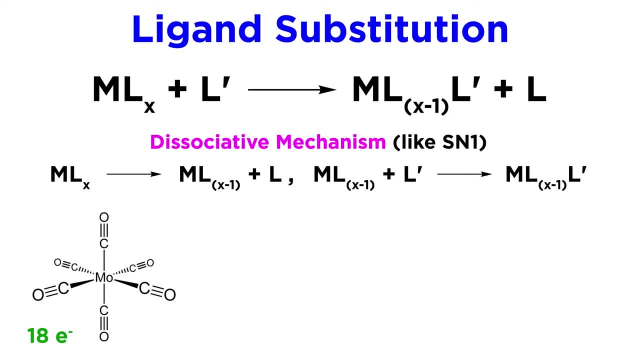 here is an octahedral molybdenum complex with six carbonyl ligands. If one of these is to be substituted with trimethylphosphine, a carbonyl will first dissociate to generate a 16 electron complex. then the new ligand will associate to restore the 18 electron count. In addition, 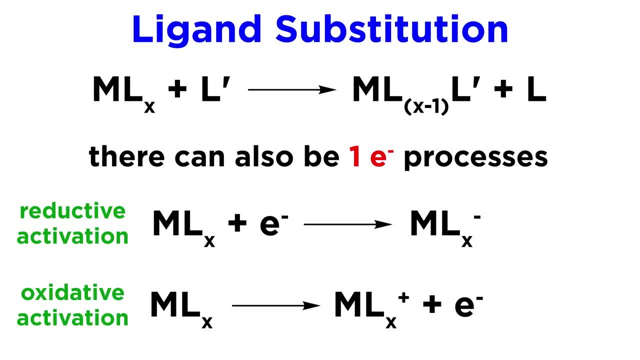 there can be one-electron processes. An activation can occur by way of oxidation or reduction, where the complex can either gain or lose one electron, thus priming it for ligand exchange. If the lumo is nonbonding or modestly antibonding, reduction is likely, while if the 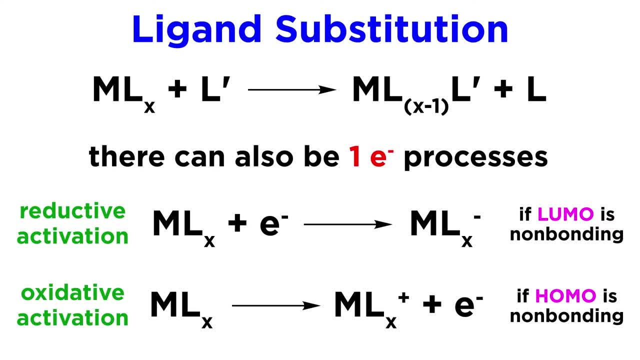 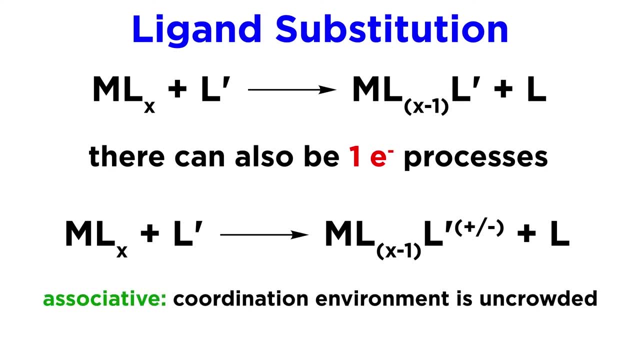 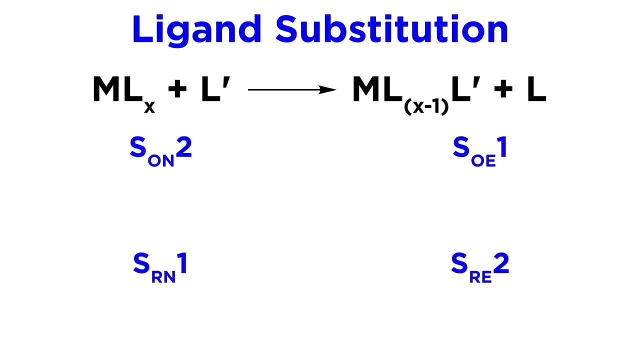 homo is nonbonding, oxidation is likely. The gain or loss of an electron can also occur simultaneously to ligand exchange, whether associative if the coordination environment is uncrowded, or dissociative- if the coordination environment is crowded, The complex can either gain or lose one electron, thus priming it for ligand exchange. If the 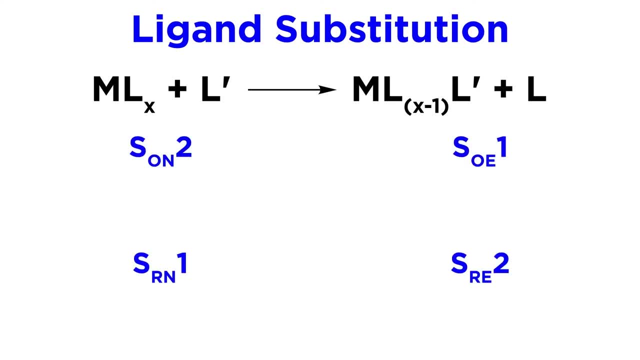 homo is nonbonding or modestly, antibonding, reduction is likely, while if the homo is nonbonding, oxidation is likely, while if the homo is nonbonding, oxidation is likely. When we combine these concepts, we can identify four common pathways. First, oxidative activation results in 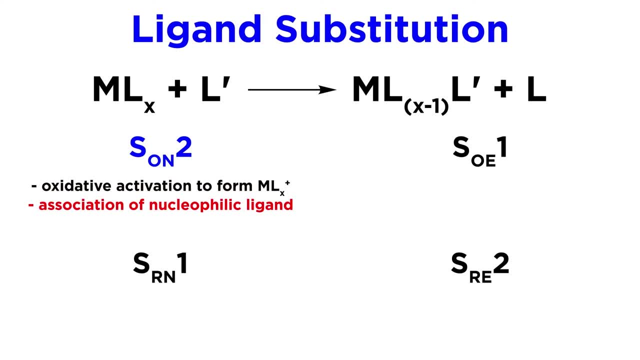 MLX+, followed by association of a nucleophilic ligand and then subsequent loss of another ligand. This is called SON2, S for substitution, O for oxidative activation, N for nucleophilic ligand and 2 for bimolecular intermediate, like the bimolecular transition state in SN2.. 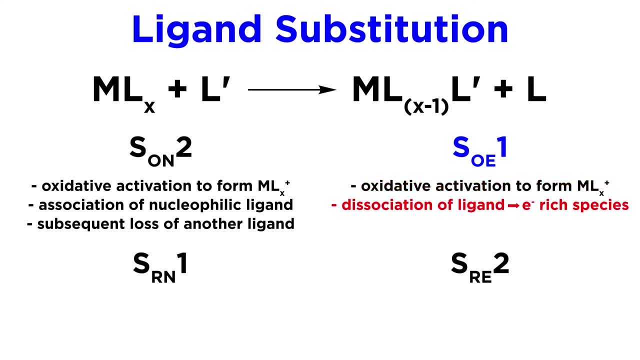 SON1 maintains oxidative activation but is followed by dissociation of a ligand to form an electron-rich intermediate and then subsequent coordination of an electrophilic ligand. So the 1 is for unimolecular intermediate, like in SN1. 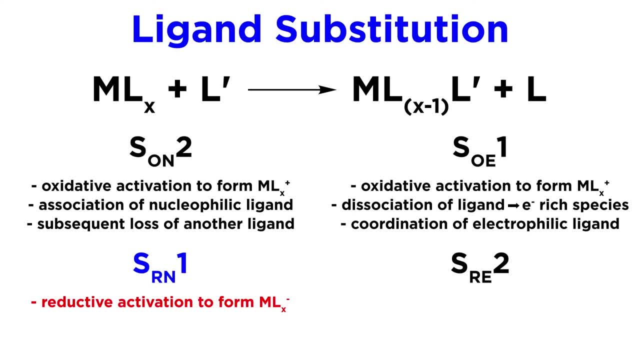 SRN1 utilizes reductive activation to form MLX- followed by dissociation of a ligand to form an electron-poor intermediate and subsequent coordination of a nucleophilic ligand. SLN1 refers to dissociation of a ligand first, then another ligand binding And lastly SRE2. 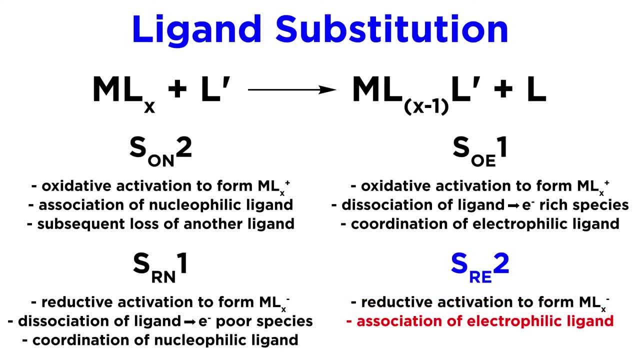 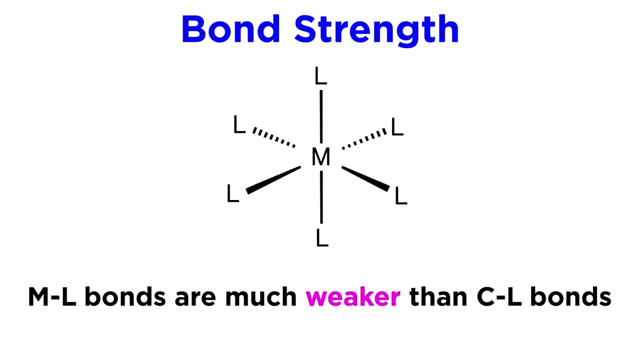 includes reductive activation, association of an electrophilic ligand and subsequent loss of another ligand. Now there is a bit to talk about in terms of metal ligand bond strength. First of all, these bonds are much weaker than those between carbon and these same ligands. They have much 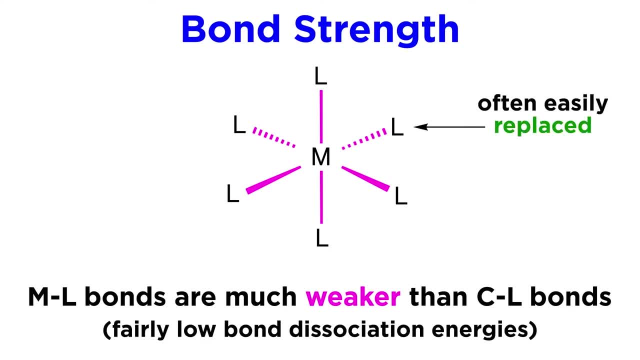 lower bond dissociation energies. That's what makes the ligand bond stronger and that's what makes the ligand bond stronger. So these bonds are fairly easy to replace and the more easily they are displaced, the more labile we can say they are. But generally speaking, these bonds get stronger going down. 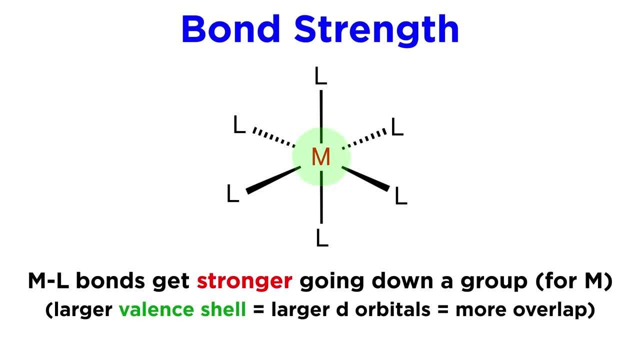 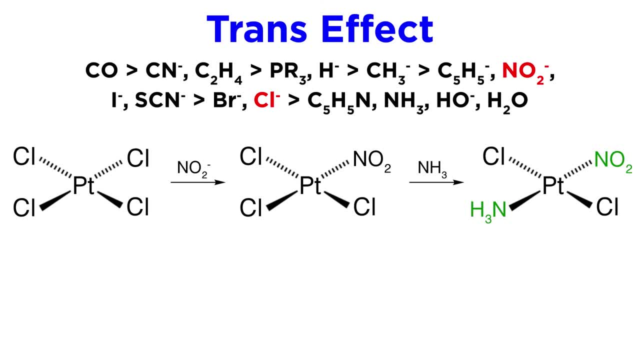 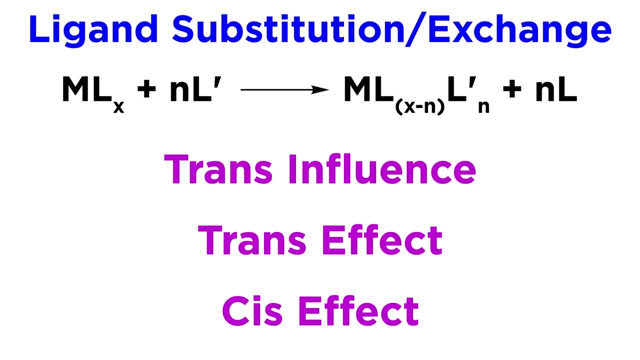 chloride. in terms of the trans effect, ammonia will end up trans to the nitrite. So that gives us a basic introduction to ligand exchange and some guidelines that we can follow to have a good sense of what will happen in any given situation. This is only the first of many. 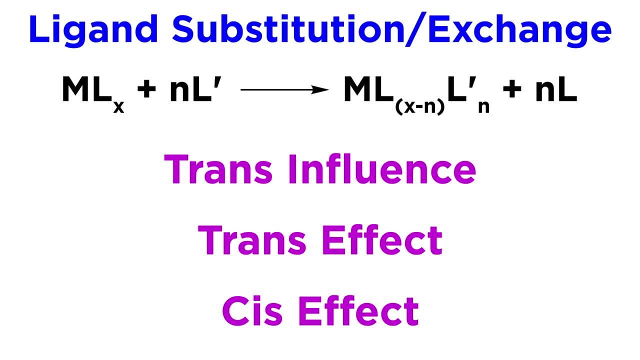 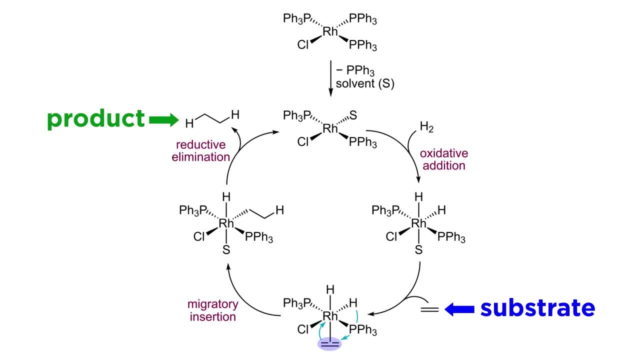 types of organometallic reactions, but it is a very important one. in catalysis, It is frequently the case that substrates become ligands on the metal in order to undergo transformation, so reactions involving ligand association and dissociation are an integral part of catalytic. 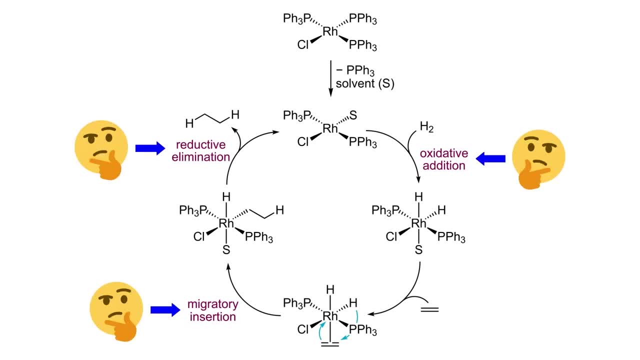 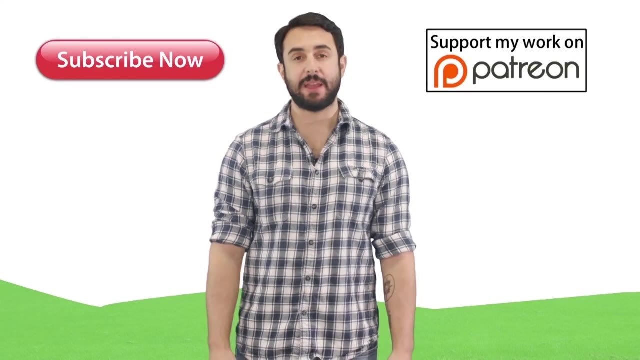 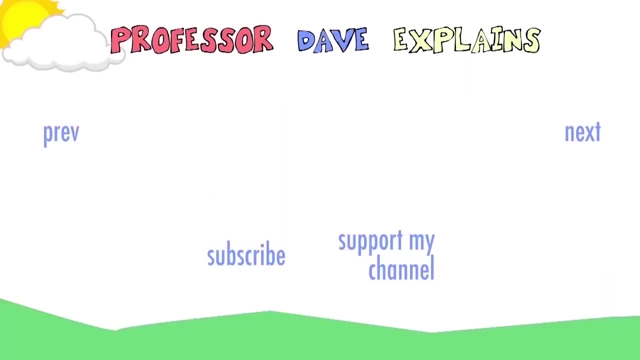 cycles. However, before we dive into the specifics of these catalytic cycles, we must continue to learn about some other kinds of organometallic reactions. so let's move forward and do just that. Subtitles by the Amaraorg community.